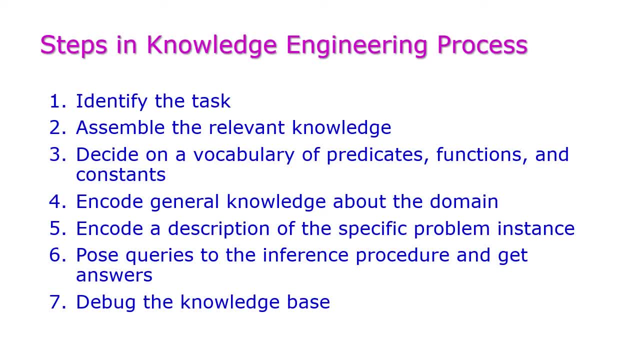 Next we will move to the important steps in knowledge engineering, And here there are seven steps. First one is identify the task, And second one is assemble the relevant knowledge. And third one is decide on a vocabulary of predicates, functions and constants. The fourth one is encode general knowledge about the domain. And fifth one is encode description of the specific problem instance. And sixth one is post queries to the inference procedure and get answer. And the last one is debug the knowledge base. Let us see all these things one by one with an example. 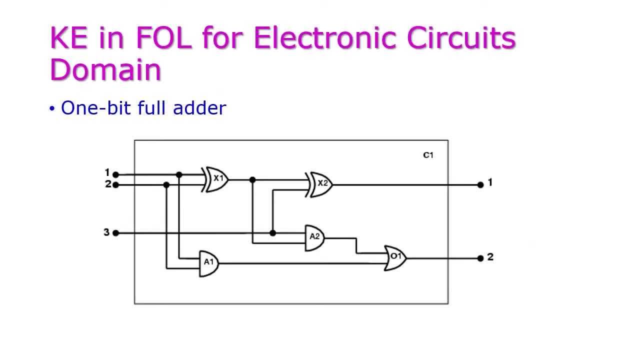 And now let us see the knowledge engineering process in detail with an example. Here we are having a full ladder circuit And this circuit is having three inputs and two outputs. Okay, with this circuit we will explain the knowledge engineering seven steps one by one. 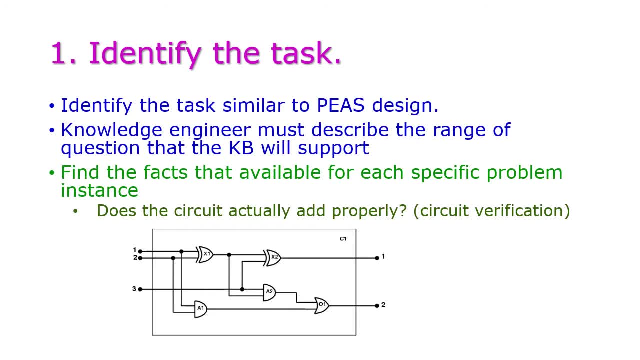 The first one is identify the task Here. identify the task. similar to piece design: Okay. performance environment activators and sensors: Okay, by using this piece. we need to identify the task And the knowledge engineer must describe the range of questions that the knowledge base will support. Okay, first we have to describe the acceptable questions by the knowledge base and find the fact which are available for each specific problem instance. 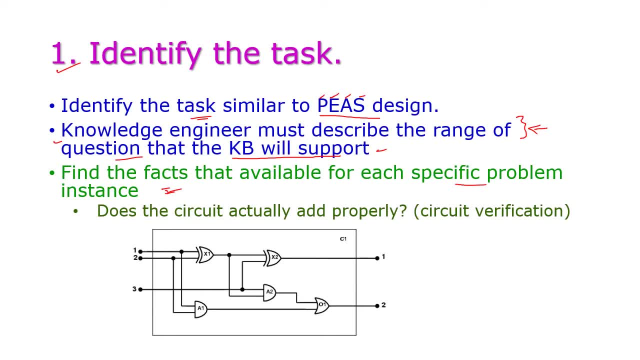 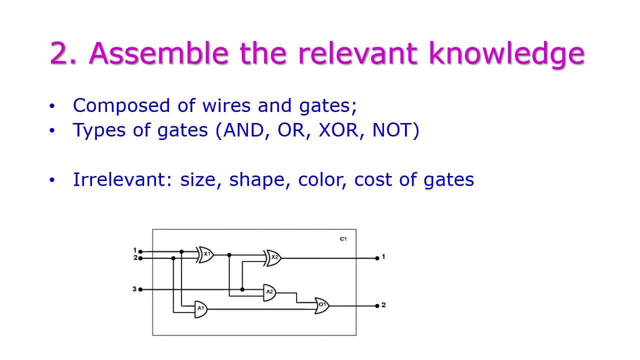 Okay, this is the task. Okay, this is the task. This is the first step Here. in this example, does the circuit actually add properly, because this is a full ladder circuit, Whether this will add all those things properly or not, we need to verify. And the second one is: assemble the relevance knowledge. Okay, so what are the relevant knowledges? are there in this domain? So here, compose of wires and gate, that is the this particular circuit. 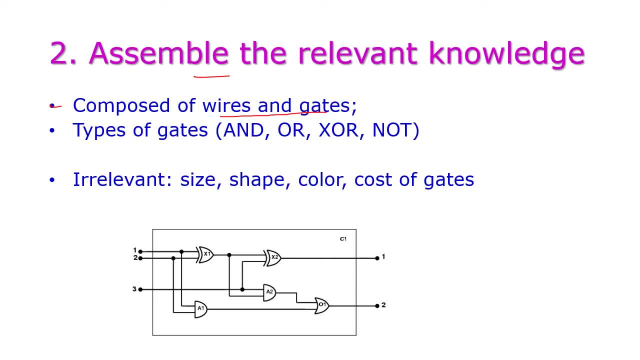 So here compose of wires and gate, that is the this particular circuit. This particular circuit is composed of wires and logical gates. So the type of logical gates are: and you get our get X, I'll get not get non-diagate, etc. So these are all different types of gates which are available for electronic circuits. 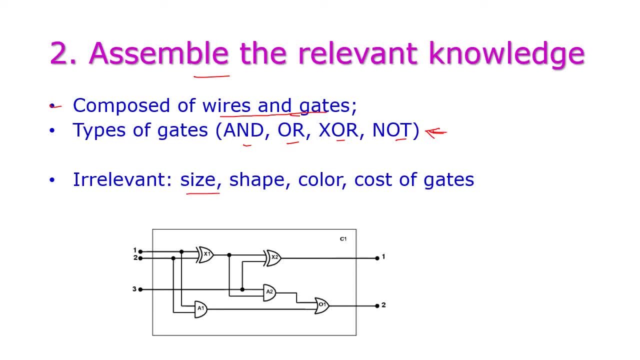 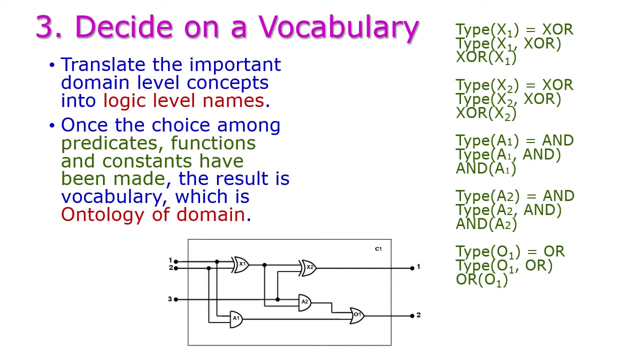 And we don't consider the properties of those circuits, that is, tallys, AP, color, cost of gate. so we don't worry about all these things. Okay, what type of gates are there And what are the truth table of those gates? We need to collect those information. So this is called as assemble the knowledge. And the third one is: decide a vocabulary, Decide a vocabulary Here. translate the important domain level concepts into logic. level names. 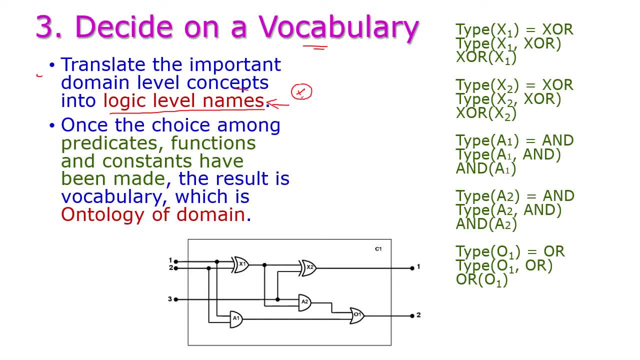 Okay, So we have to translate the important domain, level concepts, vocabularies, functions and relations and those will be converted into logic level names. And once the choice among predicate, functions and constant have been made, then the result is vocabulary, which is ontology, domain, which is ontology of this particular domain. Right? 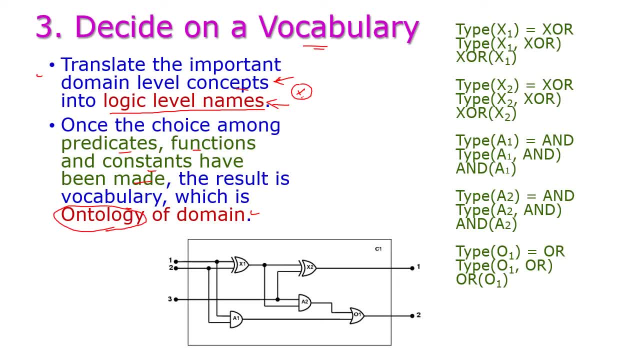 So for this example, we are having two XR gate, So XR gate 1 and XR gate 2, and two and gates, This is, and gate 1 and gate 2 and only one R gate. Okay, With these things we try to decide the vocabulary for this. First one is type of X1, which is type of X1.. X1 is XR And type of X1, comma XR and XR of X1. And like the same. 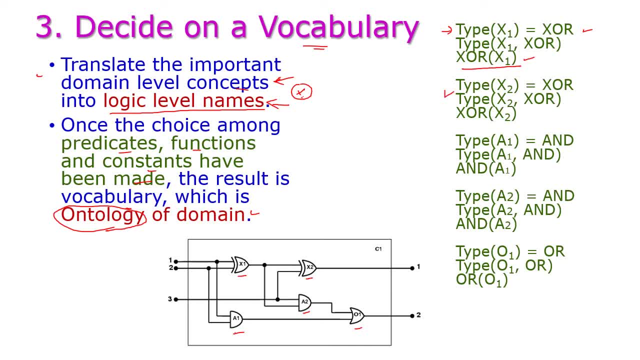 this is X1 comma, XR and XR of X1.. X1 comma, XR and XR of X1.. And, like the same type of x2, x2 is xr and type of x2, comma, xr and xr of x2. and next come to and gates, type of a1. 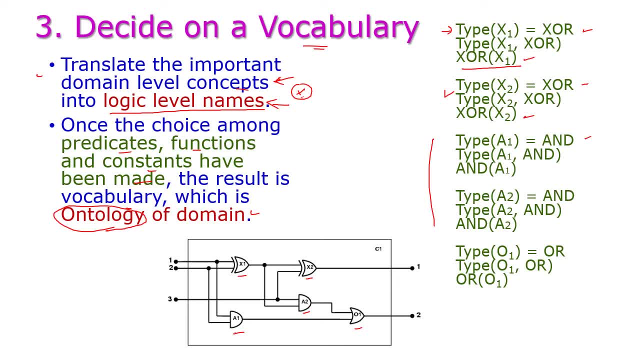 equal to and type of a1 comma, and and and of a1. type of a2 equal to and type of a2 comma, and and of a2 and type of o1. o1 is r gate, okay, type of o1 comma r and r of o1. so likewise we have to. 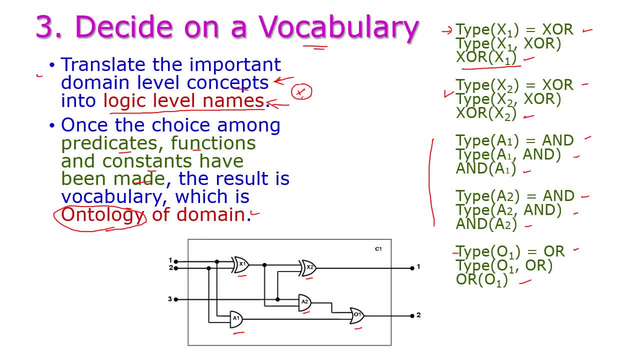 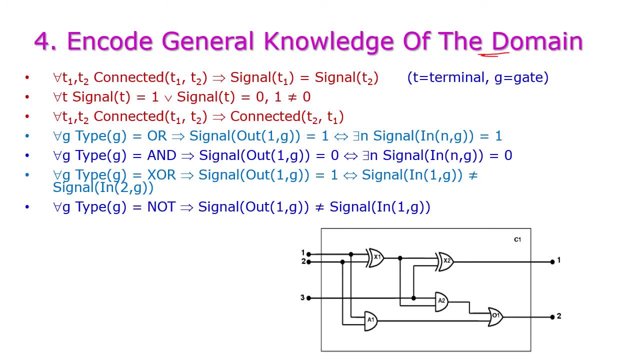 collect all the vocabularies of this particular electronic circuit. and next one is encode general knowledge of the domain. here t is nothing but the terminal, that is for all t1 comma, t2, connected t1 comma t2, which implies signal of t1 which is equal to t signal of t2. that is we are going to. 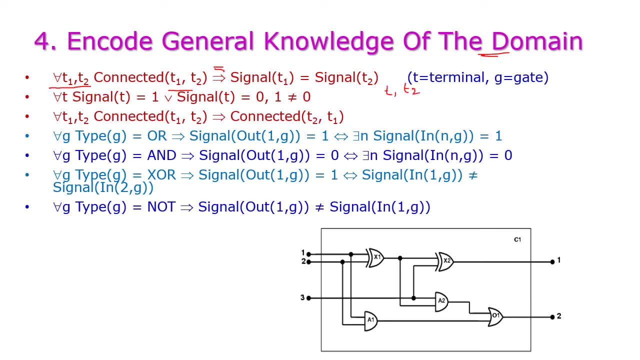 connect two terminals, t1 and t2, then the output of these two terminals will be same, right and for all. t signal of t is equal to 1, or signal of t which is equal to 0, okay, and here 1 is not equal to 0. here 0 means false and 1 means true and 1 means 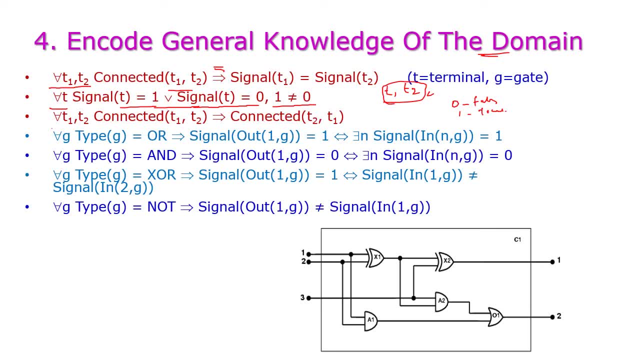 true, okay, and for all t1 comma t2 connected of t1 comma t2, which implies signal of t1 comma t2 is connected of t2 comma t1. that is, we are going to connect these two terminals. okay, then the output will be same. 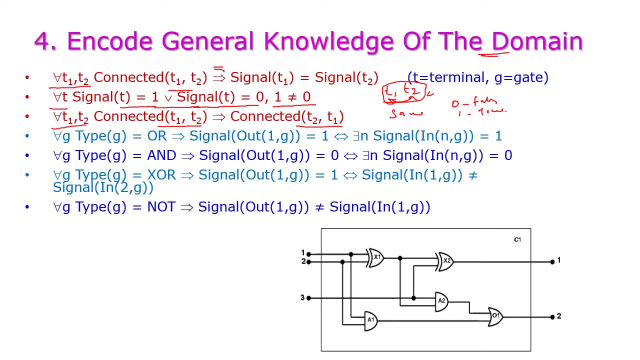 when come to r gate, right for all g. g means gate. type of g is equal to r. type of g is equal to r. okay, then, what is the output of this particular gate, that is, r gate? okay, output equal to g of t2, comma, t1. that is, we are going to connect these two terminals. 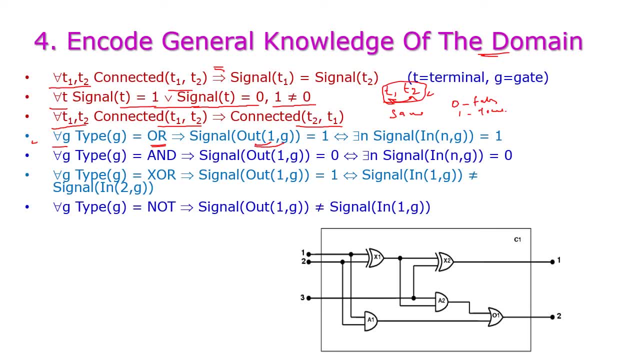 okay, this gate of signal. okay, signal is equal to 1. then there exist n input of n. okay, that is equal to 1. that means output. this is r gate. r gate output is 1, then any one of the input should be 1, then the output will be 1. okay. and when come to under gate, when the under gate output is 1. 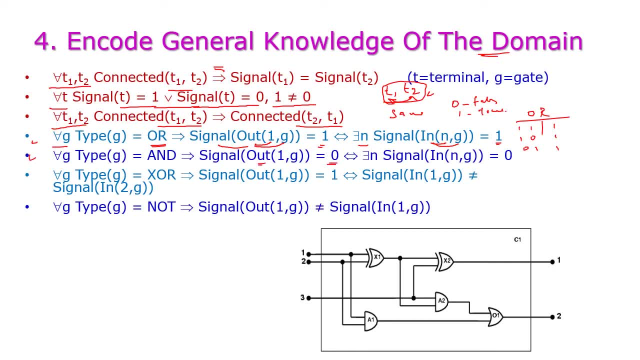 then the output will be 0. when the undegate output will be 0. if any one of the output is input is 0, then the output will be 0. okay, 0, 0, 0 here. 0, 0, 0, 1, 1, 0. if any one of the input is 0, then the output 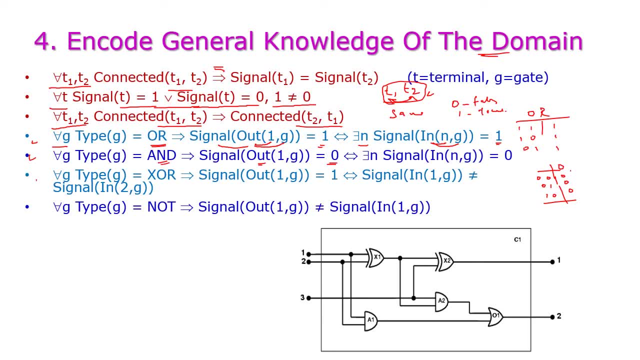 will be 0 for under gate. when come to r gate, okay, for all g type of g equal to x, r, then signal of output of 1 comma. g is equal to 1. okay, when the output of xor gate will be 1, then the input should not be equal. if we are having different input, then the output will be: 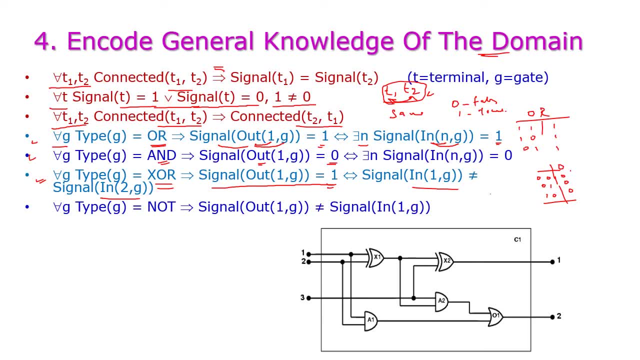 1. okay, so if two input of 0, 1, the output will be 1, or 1, 0, the output will be 1. if two inputs are same, then the output will be 0. for this xor gate, then what about not gate? if output is 1, then input. 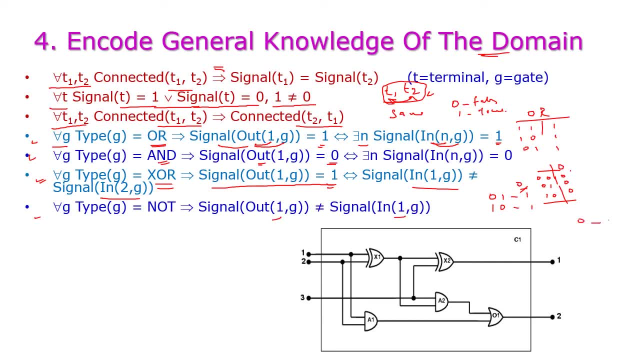 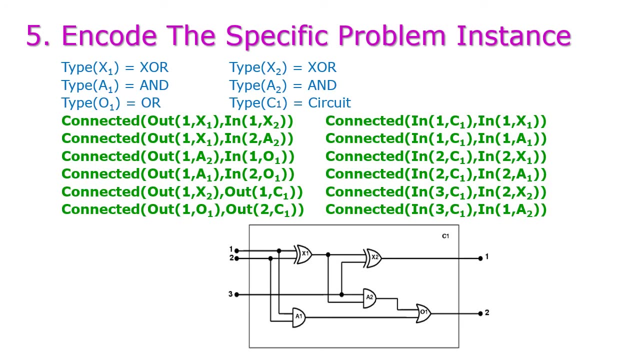 should be 0. that is, output and input should not be same for this, not gate. if the input is 0, output will be 1. if the input is 1, then the output will be 0. okay, so these are the encoding general knowledge about the domain that is the electronic circuit. here and now, let us move to the fifth. 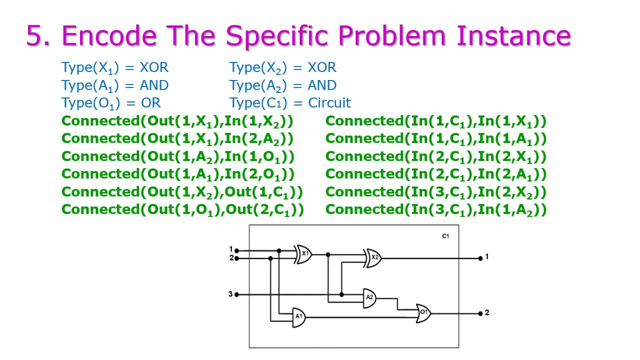 point encode the specific process problem instance. okay, here in our electronic circuit we are having five different gates. the first one is xor gate- type of gate is extra xor, and second one is xor gate and third one is and gate, fourth is also and gate and fifth is r gate and finally, 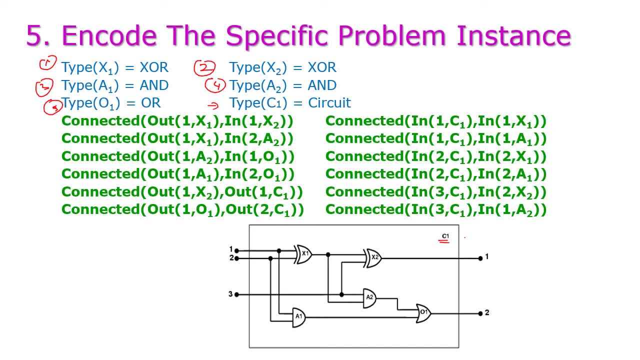 we are having the circuit c1. so in this circuit we are having three input and two output. this is c, c, c, c, c in 1, c in 2, c in 3 and c output of 1, c output of 2. this one for all the gate we are having. 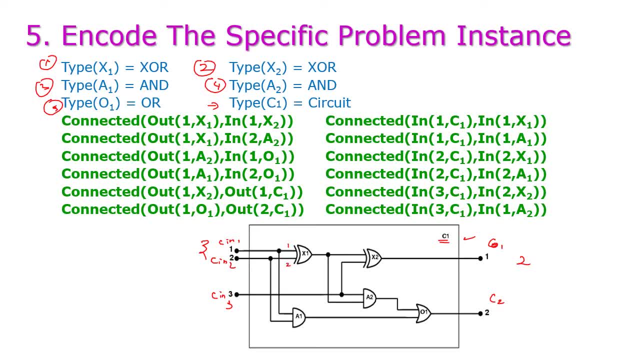 two input. this is the first input, second input and the only one output. okay, 1- 2. output is 1. input is 1. 2. output is 1. sorry, output: 1: 1. 2. output is 1. 1. 2. output is 1. okay, now let us see. 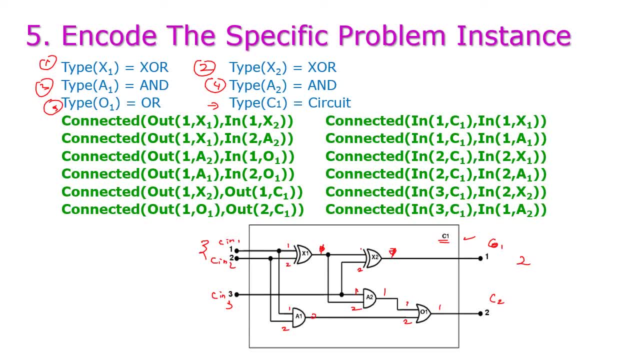 how these gates will be connected to each other. first, connected the output 1 of x1 with the input 1 of x2, the input 1 of x2. so this is: output 1 of x1 is connected to input 1 of x2. 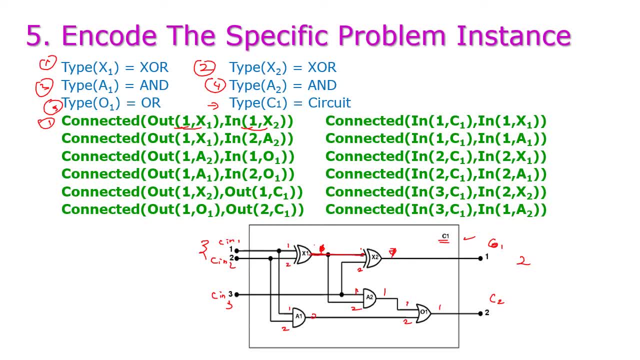 okay, this will be connected first and the second one connected of input 1 to of c1 and input 1 of x1. see c1 is here, x1 is here, input. okay, these two inputs will be connected and the third one connected of output of x1 and input of a2. so the output. 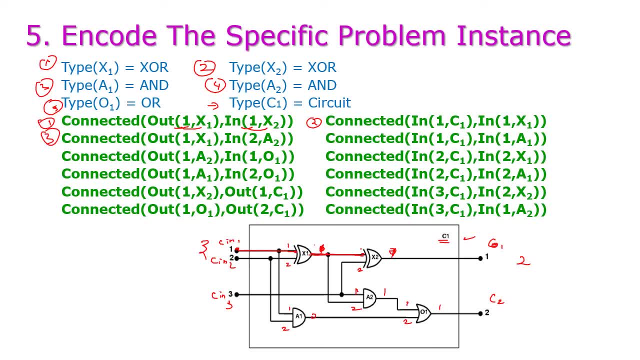 output of X1 is here and that is connected to input of A2, right, And the fourth one connected of input of C1 and input of A1. See, input of C1 is here, A1 is here. These two will be connected. Okay, And connected of output of A2 and input of O1.. Output of 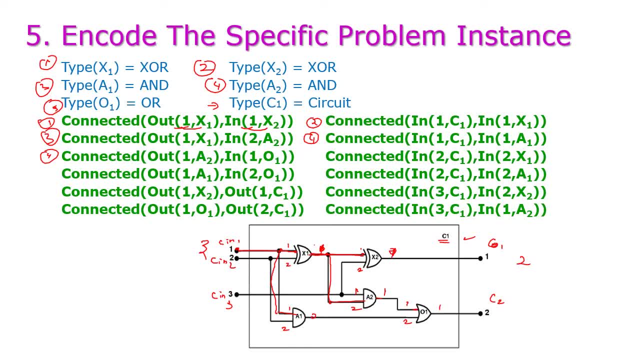 A2 is here and input of O1 is here, So these two will be connected And sixth one connected of input 2 of C1 and input 2 of X1. See, input 2 of C1 is here, input 2 of X1 is here And 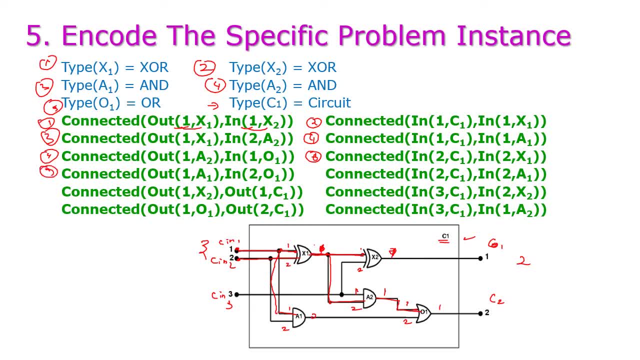 seventh one connected of output 1 comma A1 and input 2 of O2.. Okay, Connected, of output 1 of A1 and input 2 of X1. So these two will be connected And the fourth one connected. input 2 of O2 will be connected here. and next one- this is 8th one connected- of input 2 of C1. 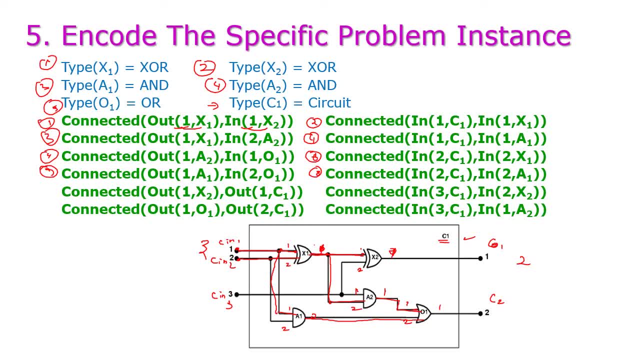 and input 2 of O1, A1 will be connected. okay, so input 3 of C1, input 2 of C1, that is connected to input 2 of O1 and the next one connected of output 1 of X2 and output 1 of C2, connected of. 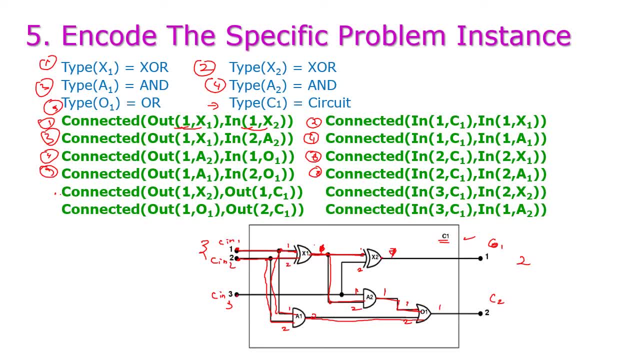 output 1 of X2 is connected to output 1 of C2. okay, this is 9th one, and the 10th one is connected of input 3 of C1 and input 2 of X2. so so so input 3 of C1 is connected to input 2 of X2. 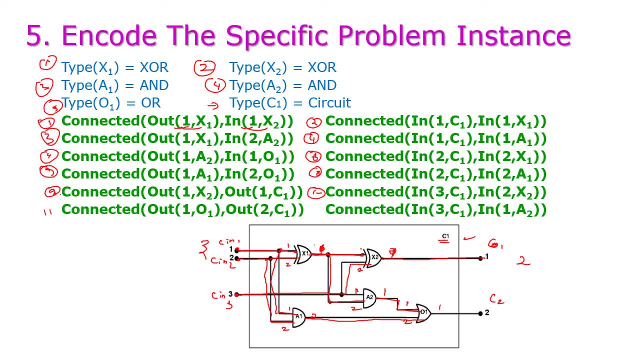 and this is the 11th one connected of: out of O1 is out of C1. out of O1 is out of C1. okay, and connected of input 3 of C1 and input 1 of A2. input 3 of C1 and input 1 of A2. 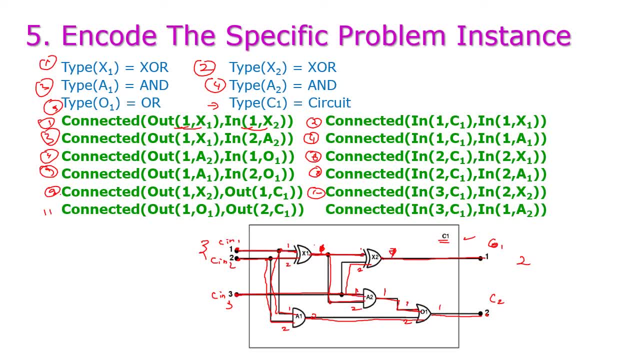 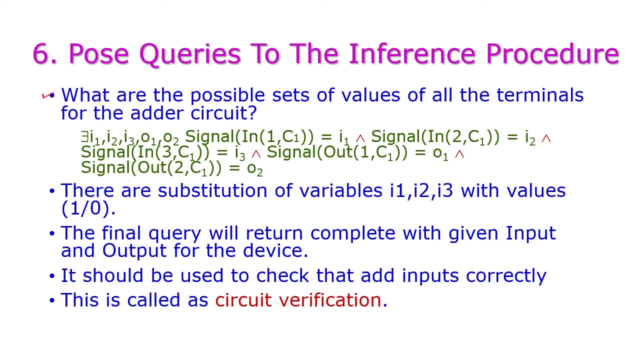 so 3 will be connected to8. so this is the 12th one. okay, so likewise we need to connect all the gates to each other. the next one is post query to the inference procedure. first one: what are the possible sets of values of all the terminals for the adder circuit here? 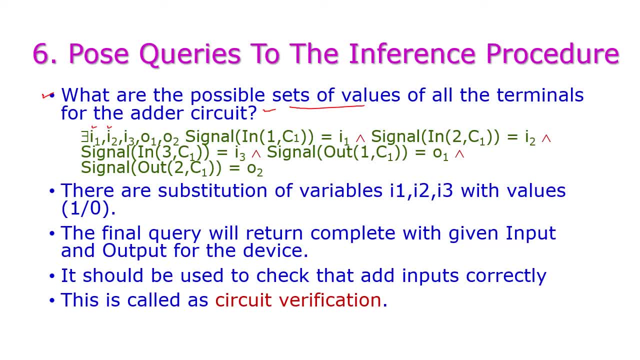 the possible set of values. there exist I1, I2, I3, O1, O2. So I1, I2, I3 are input of circuit and O1, O2 are output of circuit and signals of in of 1, C1, which is equal to I1. 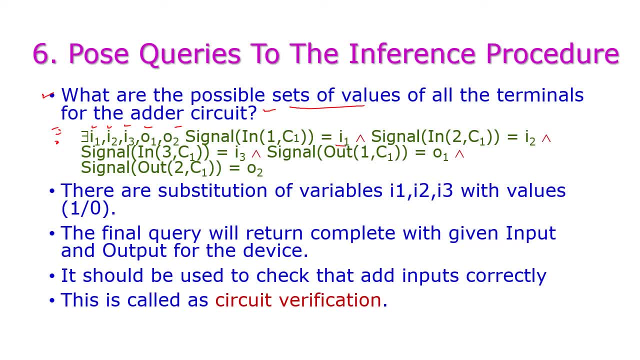 That is the first input is I1 and signal of in of 2, C1 is I2 and in of signal of input of 3, C1 is equal to I3 and signal of out of 1, C1 is O1. that is output 1 and the signal of out of 2, C2 is O2.. 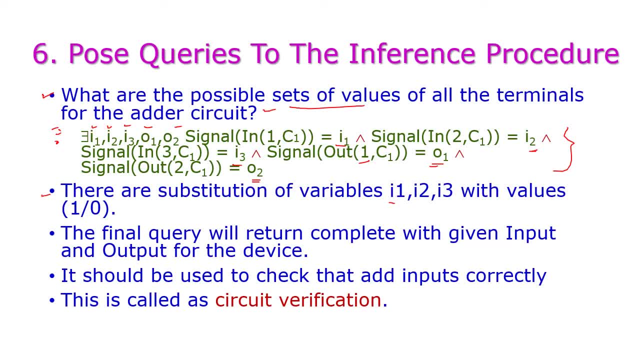 And there are substitution of circuit. So we can give the input variables I1, I2, I3 with the values 1 or 0. That is, we can give the input values 0, 0, 0, 0, 0, 0, 1, 0, 1, 0, 0, 1, 1 and 1, 1, 1, 0, 0. 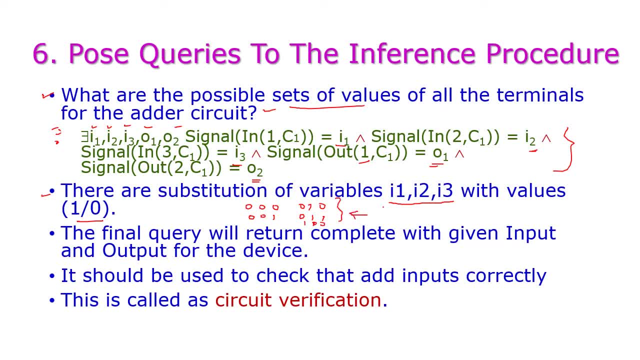 So likewise we can give the possible of input combination of input to the circuit input values And then final query will be written to complete With given input and output for the devices And it should be used to check that add the inputs correctly or not. 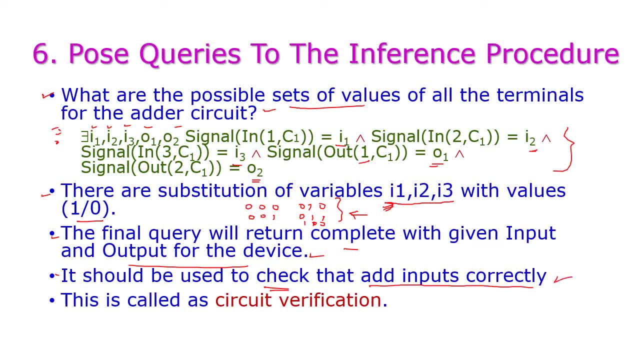 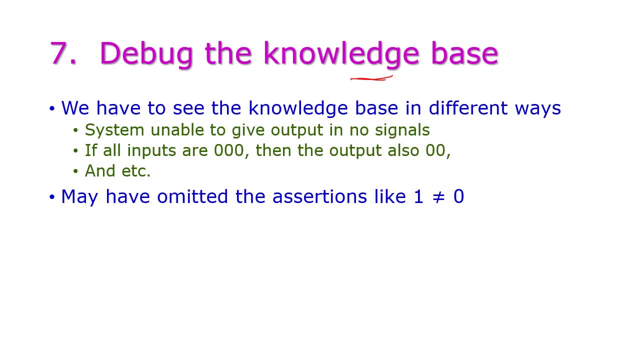 Because we are giving all possible values to the input, then we need to test the output, whether these two are correct or not, And this is called as circuit verification. And the last point is debug the knowledge base. So, once all the possible inputs will be checked and verified,